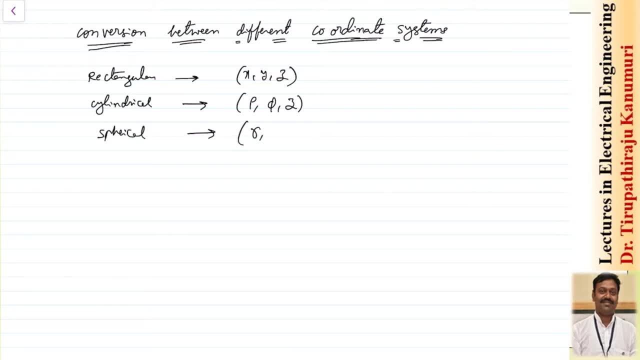 system, the sphere is represented by the radius and the value of theta. This is with respect to the z axis and phi. These are the coordinates. So let us see how to convert from one coordinate system to another coordinate system, For this simple thing is there. let us take, for example, 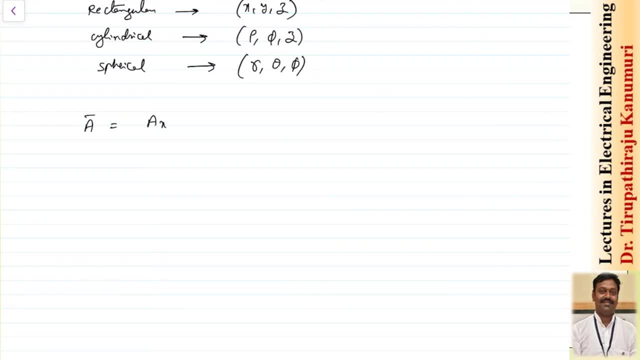 I have a vector a. Let us assume it is a rectangular coordinate system. It can be any coordinate system. Other can be done in the similar way: Ax in the direction of x, Ay in the direction of y and Az in the direction of z. So this I want to convert to: 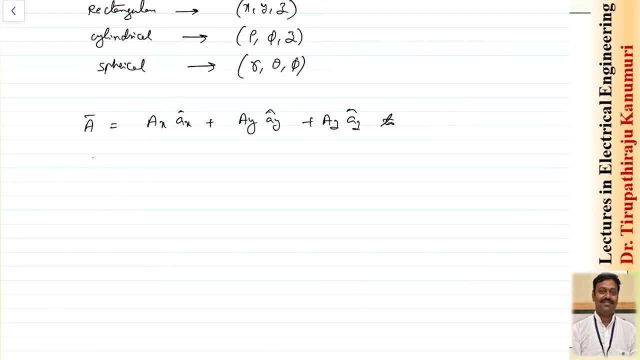 let us assume I want to convert to spherical coordinate system, for example. So spherical coordinate system, we know the components are a, This will be r in the r direction. So similarly, there will be theta direction will be there. Let us take it as theta. So similarly. 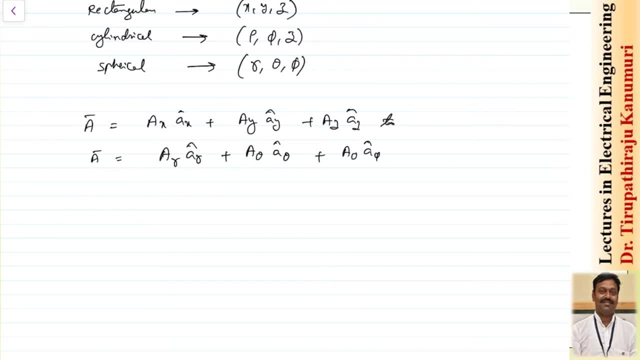 third component will be in the phi direction, So that is why let us take it as phi. So I have to convert this one into this format. So, in order to convert this to this format, you needifice coefficients, because unit vectors are having unit magnitude. There are no issue. 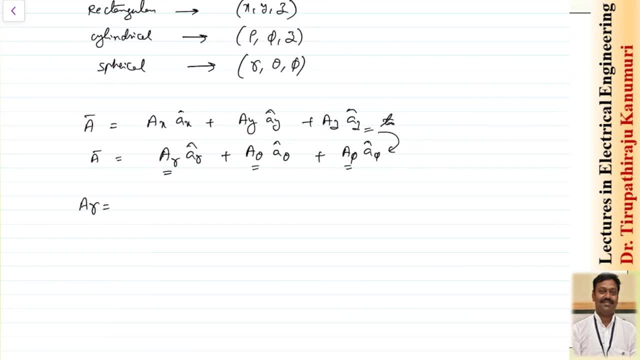 So to calculate this value of each one, This is nothing but the scalar projection of this vector a in the direction of r. So this will be a scalar projection of a in the direction of theta. It will be this one, a theta. Similar is the case for phi. How to do the scalar projection, We have already. 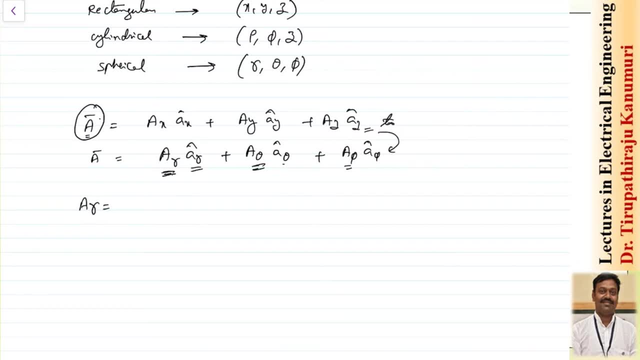 seen the dot product or how theippiolar projection can be done. So this can be done by taking BMW TWO product of a in the direction of r. So you want a r, So just take the dot product in the direction of r. So what will be? what does this mean? This will be a x. This unit vector a, x will be dot. 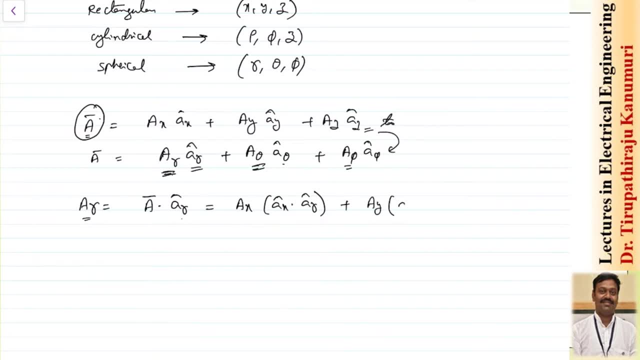 product with a r. Similarly, this will be a y. This a y will be in the dot product with a r. Similarly, a z. This will be a z will be dot product with a z. Similarly, if you want to calculate, for example, a theta, a theta will be a dot product with a theta, So this will be a x. 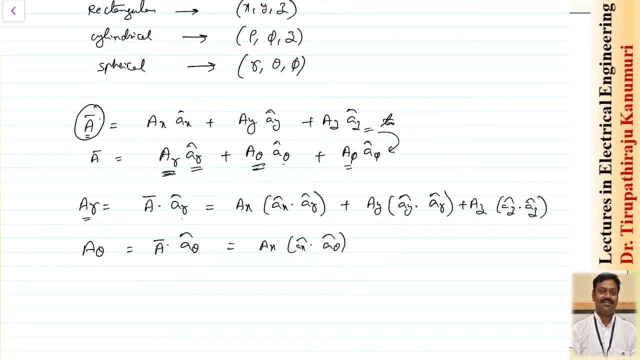 into a x dot product with a theta. Similarly, this will be a y. this will be a y dot product with a theta. And this is third component, that is, az dot product with a theta. This way I have to calculate. So same way I can calculate for the phi. So this will be equal to a dot product with. 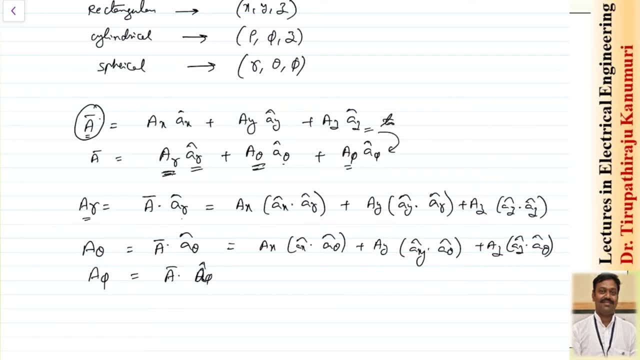 phi, a phi, unit vector phi. so in this way i can calculate, so let me just erase this. a phi, so in this way i can calculate it. so for calculating these things, because in order to calculate the ar, a theta and a phi, i need the dot product. so this product, if you know the table, 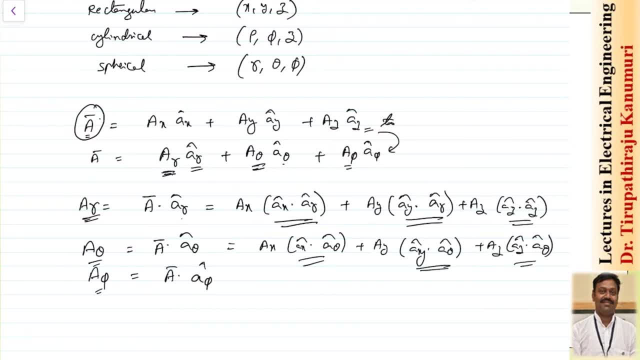 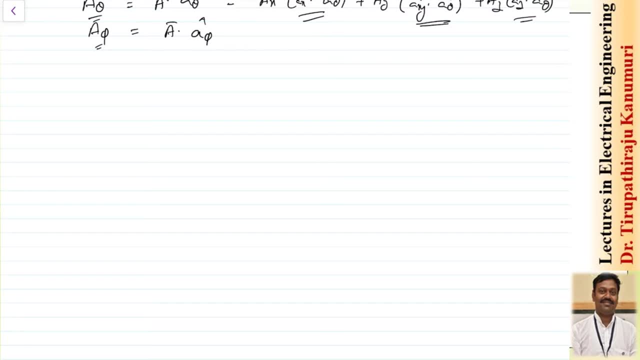 then you can do the conversion very easily. so let us see how to convert between the coordinates, for converting from between the coordinates, or to know this table. first let us briefly discuss about different coordinate systems. if you take the rectangular coordinate system, it will have three coordinates which are perpendicular to each other. this will be x, y and z. these are: 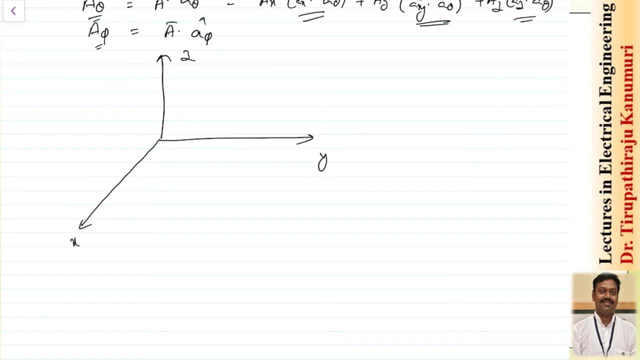 perpendicular to each other. now, if you want to represent any point, so that point will be represented by how much it is shifted in the x direction, then how much it is shifted in the y direction, followed by how much it is shifted in the z direction. so this will be my point. let us 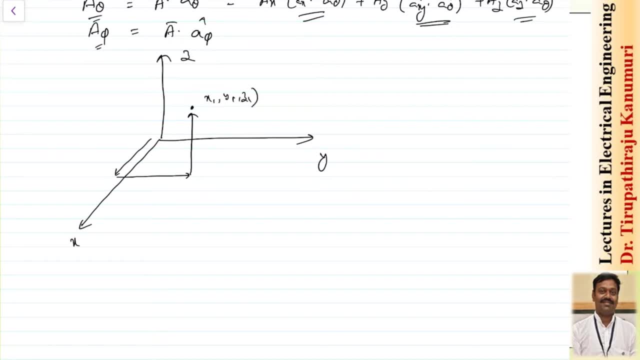 assume this is x 1, y 1 comma, z 1. how this is obtained by shifting in the x direction, shortly y direction and then followed by the z direction. so using this i will get the values. so these are represented by x1, y1 and z1. so let us see the cylindrical coordinate system. then we will see. 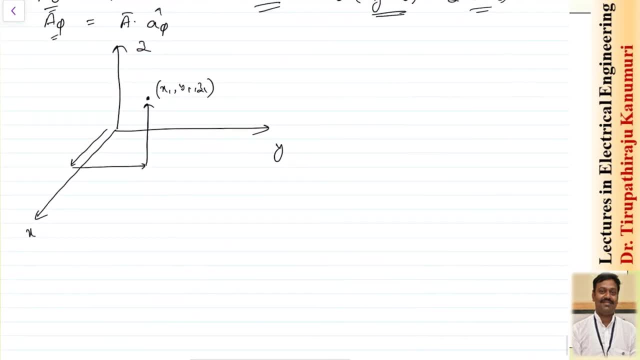 the relationship between these two. so in the cylindrical coordinate system, again, x is here, y is here and this is my value of z. in cylindrical coordinate system, first thing is that using the x and y coordinates we form a circle. so let us take, for example, i have a particular value of x. 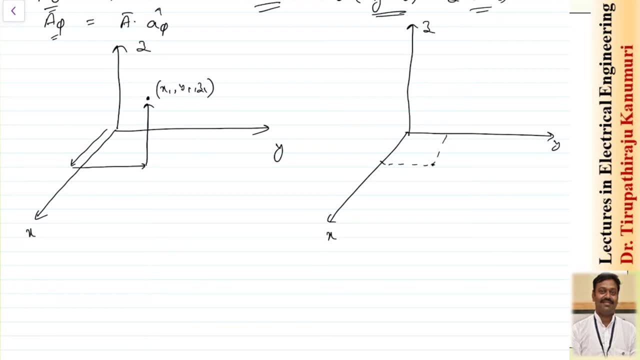 so, similarly, i have a particular value of y, so this point came. so this: in the xy plane this is called as. this radius in the xy plane is called as rho. this rho will be equal to square root of x square plus y square. so let us assume it is making an angle of phi with respect to your x axis. 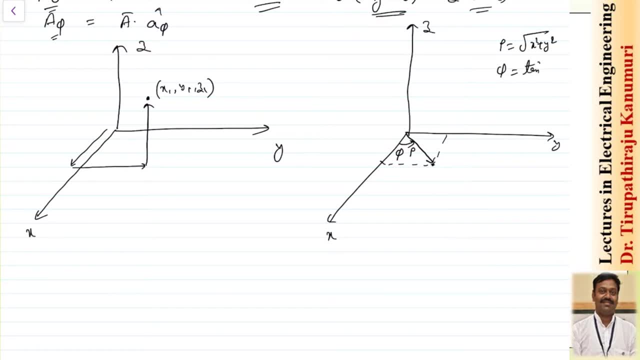 this phi i can obtain by tan inverse of opposite, by adjacent. so tan inverse of y, by x or otherwise, the rho in the x direction gives the x component. so we can calculate: the x component will be equal to rho, cos phi and y will be equal to. 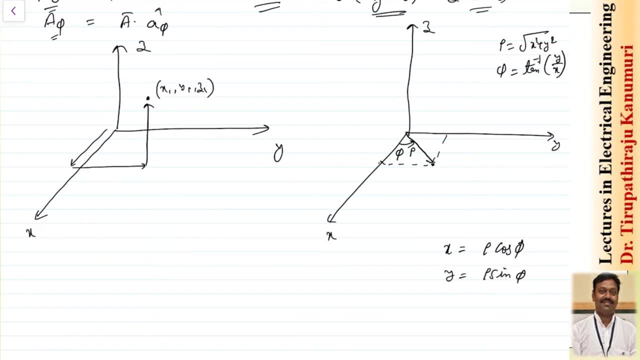 rho sine phi. this is the relationship between these two. now to this row. using this row, that means by varying the value of x and y- i can maintain the row value constant. if you maintain the row value of constant by varying different values of x and y, you will get a circle. so let 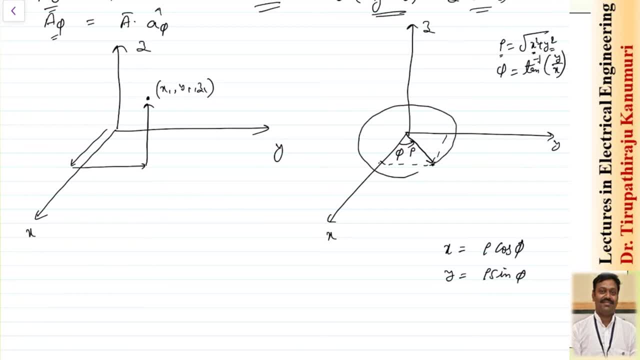 us assume you got one circle like this. you got one circle. so now if this circle is projected up in the dimension so that leads to the cylinder, a cylinder will be formed there. so how much? it is projected from here in the vertical direction. so this gives my point. let us assume i want to find some. 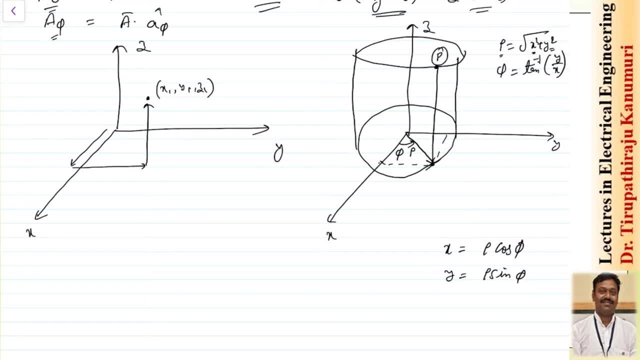 particular point. this is my point p. this point is represented by what is the value of rho and what is the phi, what is the shift with respect to x axis and what is in the z axis getting it, how the cylinder will be formed. let us see how the conversion takes place between different coordinate systems, so that i am 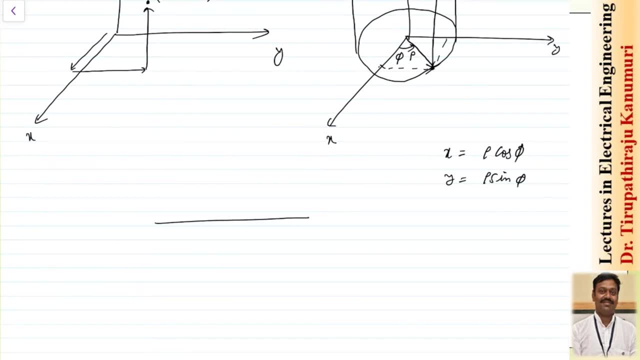 again drawing this cylindrical coordinate system. so y, x and z, so let us take the half part so that it will be easy to analyze. so i am taking this one. so i am taking a, say, quarter part of a cylinder. that means one fourth part of a cylinder. so how? 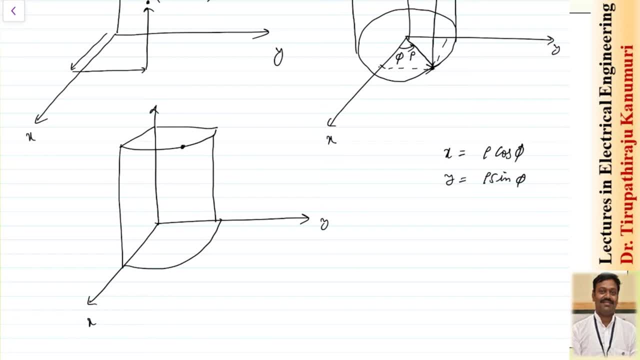 it is coming. so let us assume one point is here. so to reach this point, how we will get? just project it onto the x, y plane. it is intersected at this point. so this indicates my value of rho, this indicates my value of phi and this height indicates the value of z. so at this point, this: 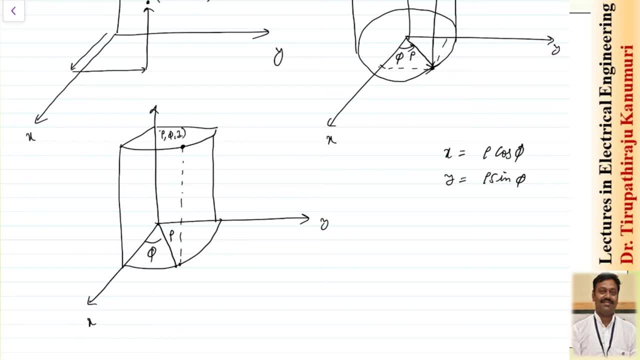 will be equal to rho phi and corresponding value of z. corresponding value of z means when your project is to the z axis. this gives my value of z getting it. so at this point let us see how the different components will come. if you are varying the value of the row, row will be: incremented in this direction. this is my direction of arrow. or if you are for adding a value of this, we will attract that value of that as well. the on the second value, max merchandise value will be equal to i. since i am trying to apply height value二 equal to two, do not enter都いただ以. 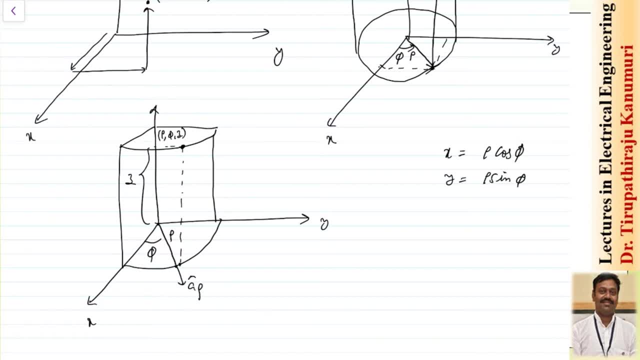 Or I can tell that rho will be in the incremental direction of this radius. This is my value of A rho. Similarly, phi will be in the incremental direction of phi, because phi is taken with respect to x axis. This will be my direction of A phi. 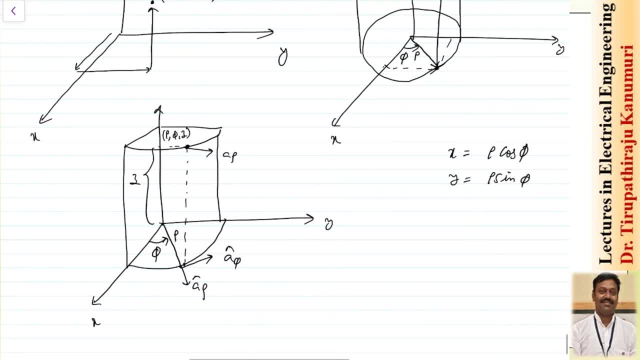 And similarly, if you want to take the z direction, z direction will be: z will be incrementing in the direction of z. This is my direction of A z. So let us see how to resolve each of these components into the x, y and z coordinates. 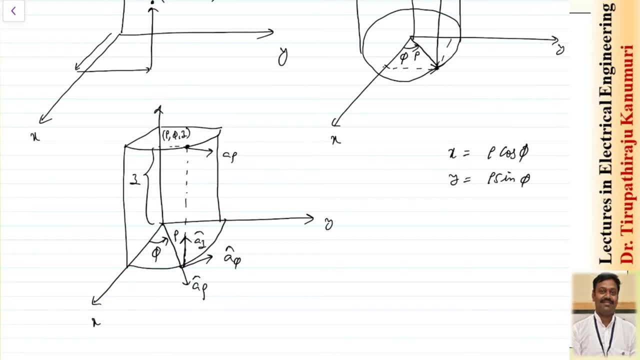 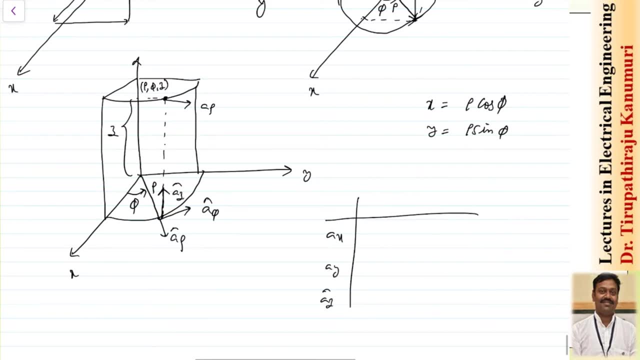 or vice versa. So let us see one by one. So for that, I am just preparing a table. This table I am preparing between A x, A, y and A z. Remember the dot product is commutative. 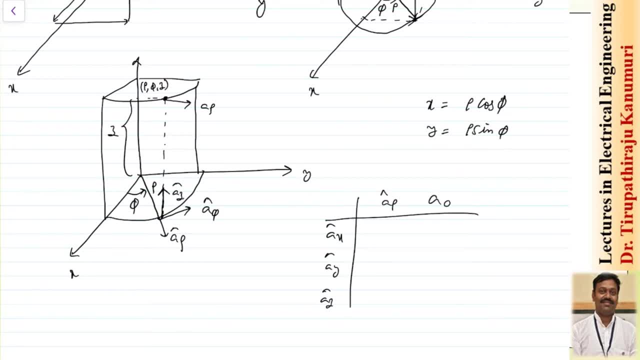 So there will be no difference, even if you are reversing A phi and A z. So let us take A rho. This is my value of A rho. This A rho I can project in the direction of x. How to get it? 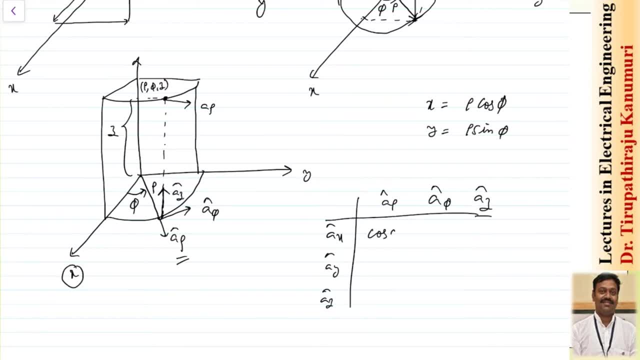 By taking the value of cos phi. So this is my value: is cos phi? Similarly, y y will be equal to y. y is this component. Our y component will be sin phi. Remember in the exam: if you can visualize your coordinate system properly, you can derive. 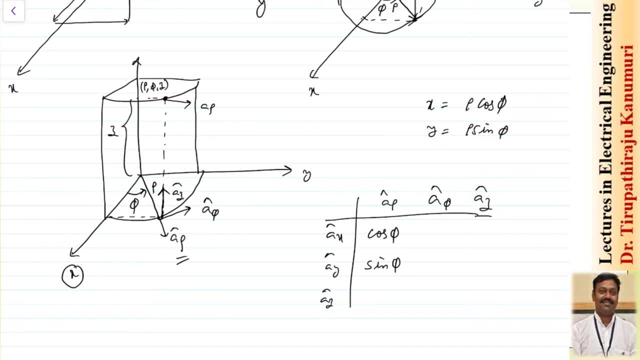 this table there directly in the exam, No need to muck up anything. So similarly, A, z, Because rho, phi and z are the three coordinates in cylindrical coordinate system. Both are 90 degrees perpendicular to each other. So obviously z component will be equal to 0, because cos 90 is equal to 0. 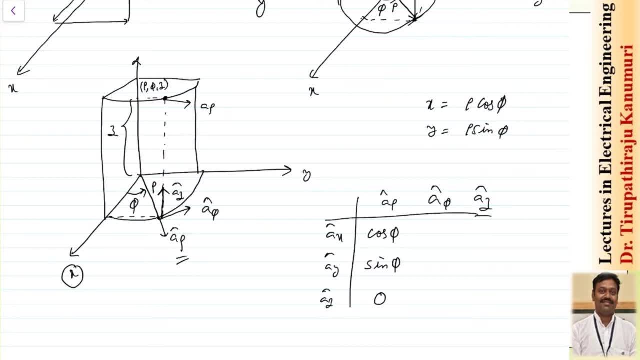 Now let us take the z component z you can see here. z is in the rectangular coordinate system also. That means in rectangular coordinate system. z is in the rectangular coordinate system. So in this system A x and A y are 90 degrees perpendicular to A z. 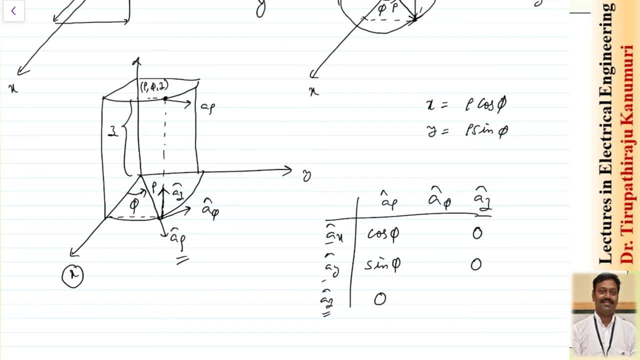 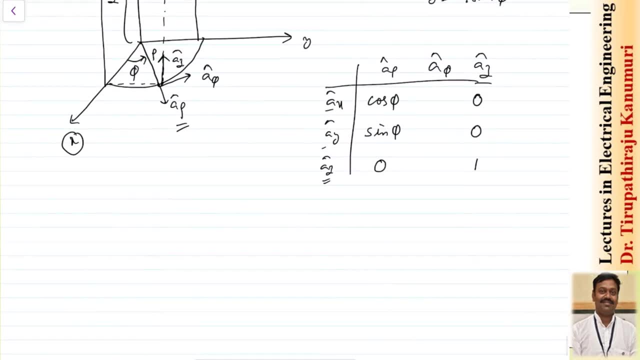 So automatically, cos 90 will be equal to 0.. Only A z dot product with A z will be equal to 1.. So z is over. Now let us see how to calculate the value of phi. So to calculate the value of phi, I am simply taking my x coordinate and y coordinate. so 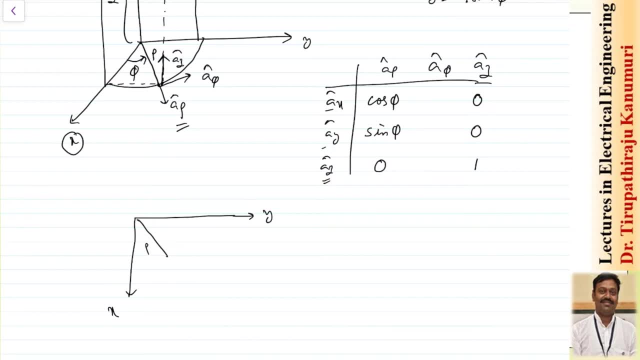 that it can be visualized easily. So let us assume this is my value of rho, This is my value of phi. So incremental value of phi will be tangent at this point. So tangent, I am just extending. I can extend like this: 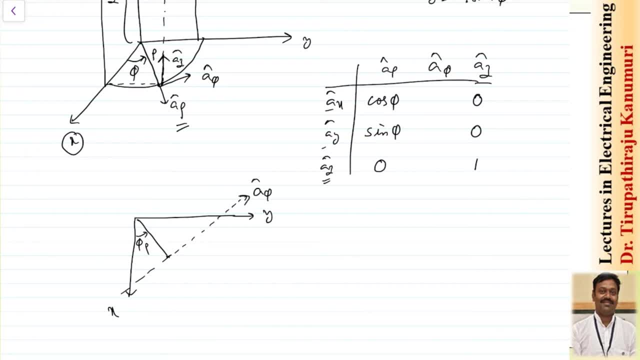 This is my value. This is my value of A phi unit, vector phi. So this angle is 90 degrees. So this will be equal to. because total angle is 90 degrees, this will be equal to 90 minus phi. 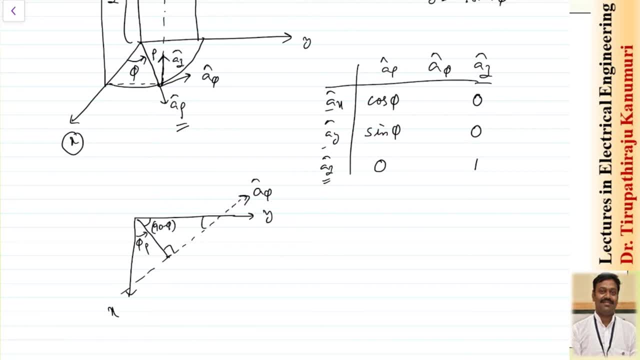 If this is 90 minus phi, because this total sum in this triangle will be 180 degrees, this will be equal to phi. So obviously this will be equal to phi by symmetry. So this A phi has two components. One component is in this direction. 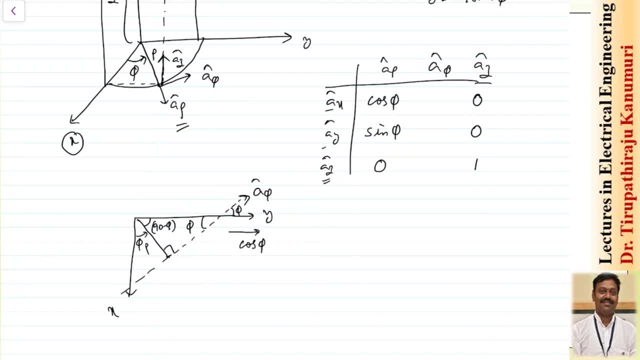 So this can be obtained by taking cos phi. Second component will come in this direction. This will be obtained by using sin phi. That means we can tell that the sin phi is giving opposite to the direction of x. If you want in the direction of x, I have to take the minus sign. 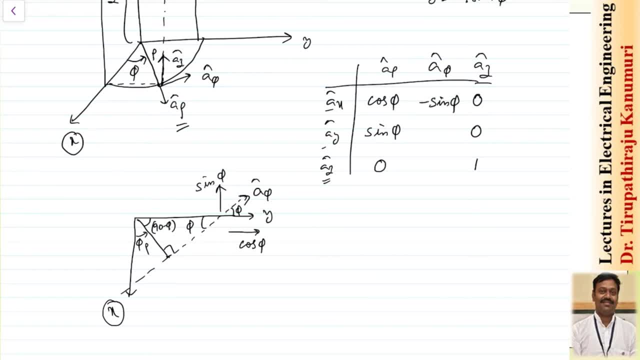 So that is why this will be equal to minus sin phi. Similarly, if you want, in the y direction, y direction can be obtained by cos phi. Now coming to the z, Because we know the phi is in the xy plane. it is 90 degrees perpendicular to the z plane. 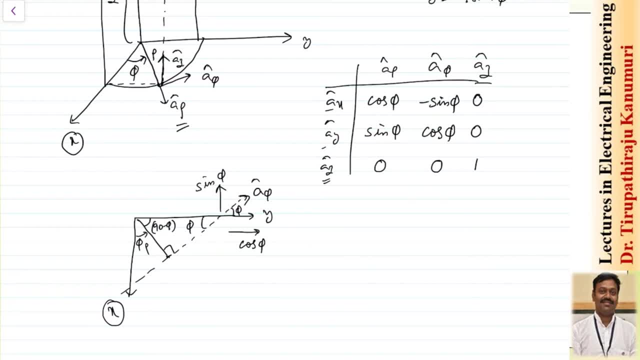 So obviously the dot product with the z will be equal to 0.. So this is the way how to convert between rectangular to cylindrical coordinate system and cylindrical to rectangular coordinate system, vice versa. So using this, we can do the conversions. 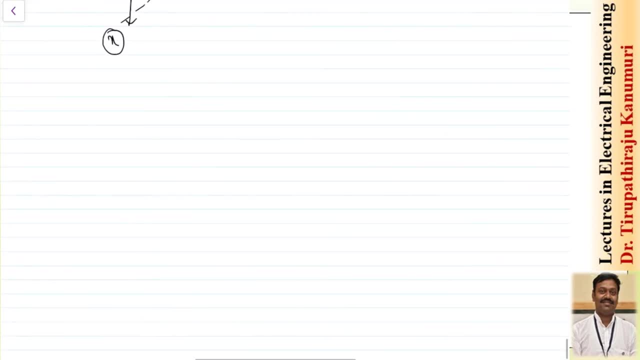 So let us see what is the spherical coordinate system. How does it comes So, for knowing the spherical coordinate system, Let I assume I have one sphere. So let us take the coordinates. This is my x coordinate, y coordinate and this is my z coordinate. 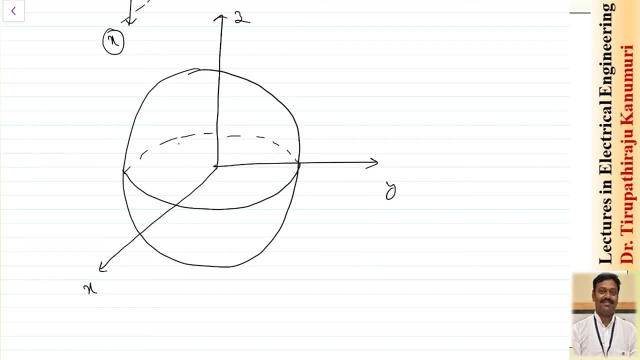 This is my value of a sphere, Getting it. so in this pair, let us assume i am taking a small arc, so a particular line, so let us assume it is varying like this, so in this line, some particular point i want to represent. this is my point p. 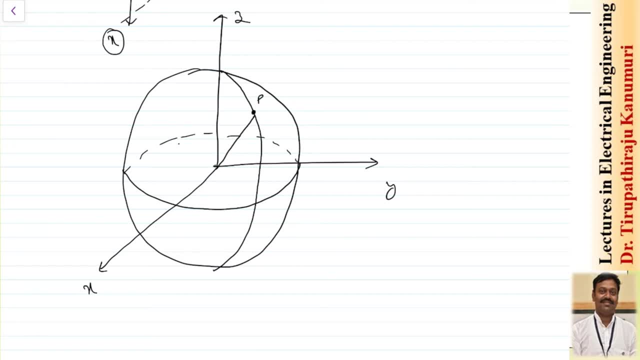 generally, this point is represented by the radius. what is the length? so this is equal to radius. and what is the angle with respect to z axis? this is given by the value theta, the angle with respect to z axis. and the third one is when you project this to the x y plane. that means when you project. 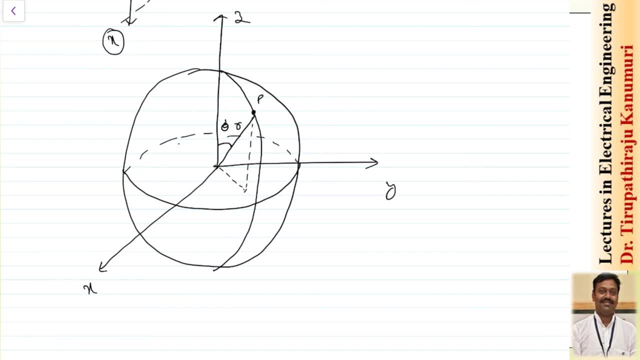 this point to the xy plane, so this point will form an angle of phi with respect to the x-axis. that means when you project this point to the x? y plane, it will form an angle phi with respect to x-axis. so this length i can consider as the value is rho getting it. so this way these are: 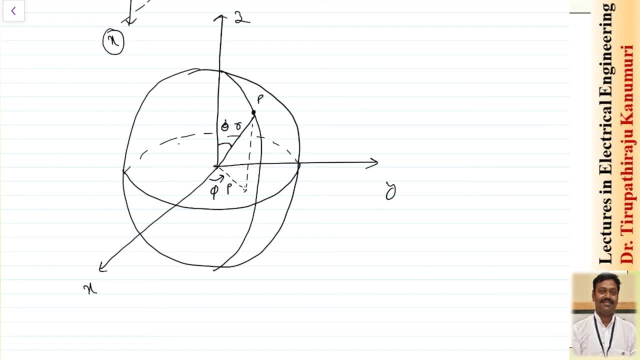 the three coordinates. that means the three coordinates in this spherical coordinate system are r, theta and phi. these are the three coordinates. so now let us see what are the lengths of various coordinates here. so this length will be, if you are projecting this in the z-axis direction, so this will become equal to: 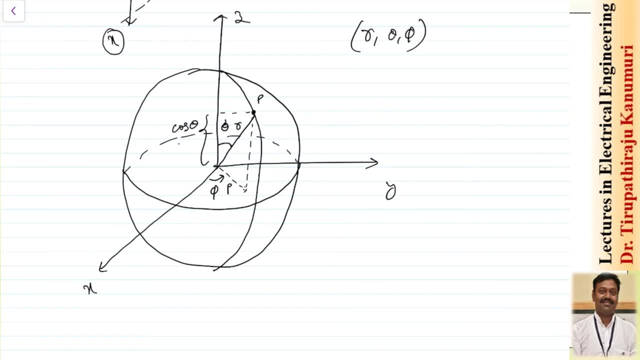 cos theta. That means r is projected in this direction. r cos theta. Similarly, this projection or the row will be equal to r sin theta. This will be equal to r sin theta. Remember this much basic, so remaining things we will see. So now coming to unit vectors, because in order to get 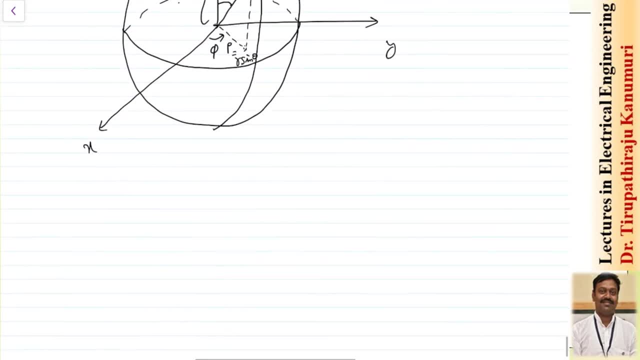 the table. we need the unit vectors. So let me draw the table first, then after that we will give one by one there. So for this coordinate systems, let us take between cylindrical and spherical coordinate system first, because it is easy. After that we will go for remaining. 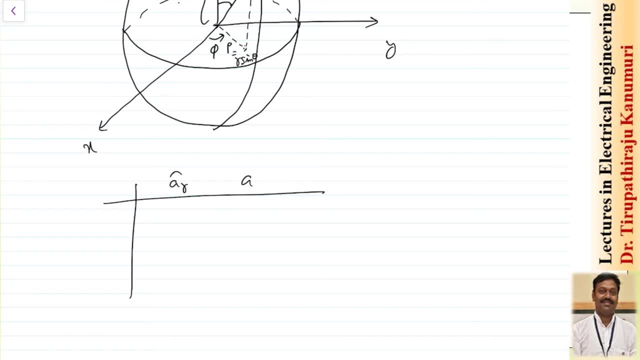 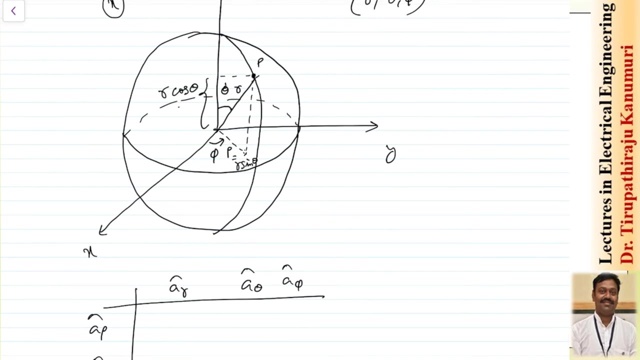 coordinate systems. So let us take it as ar, a theta and a phi. So here I am taking a rho, a phi and az. here You can do the vice versa, because it is a dot product, only Now coming to the ar. So generally the value of ar, the unit vector ar, will be like this: 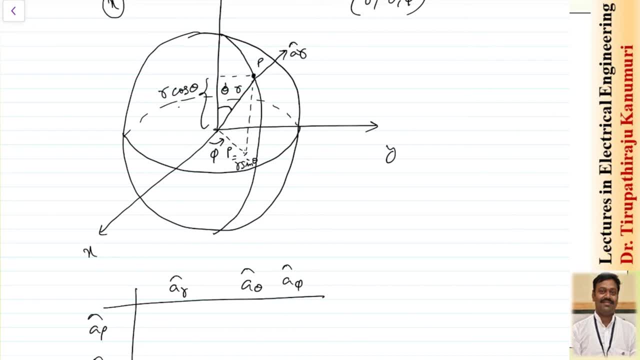 incremental direction of r And this will be my value of the rho. incremental direction of the rho. it will be in the xy plane. That means if you want to convert r to the rho then it will be equal to you have to project. 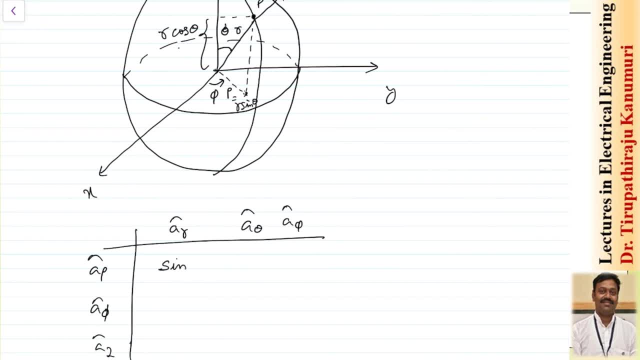 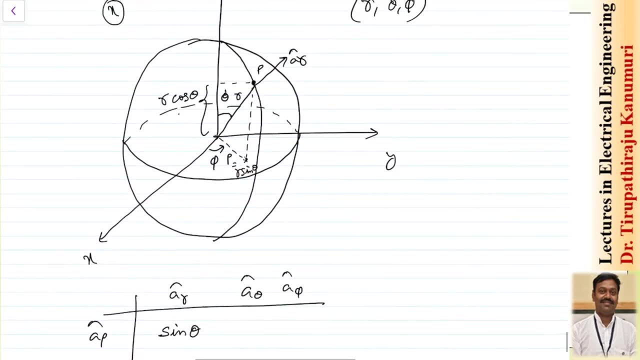 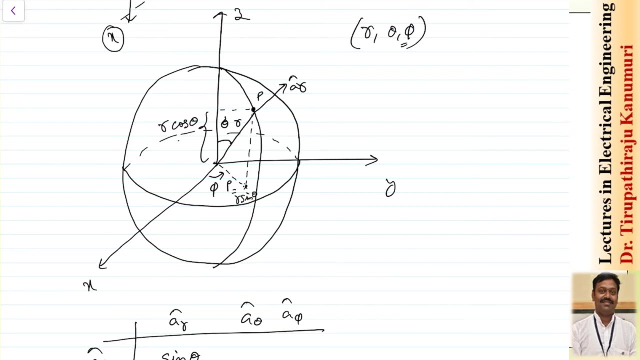 this to this side, So it will automatically equal to sin theta. ar in the projection of this will be equal to sin theta, Then ar in the direction of phi, because phi is there in this coordinate. also automatically, this is perpendicular to the value of phi, because the value of a phi will be like: 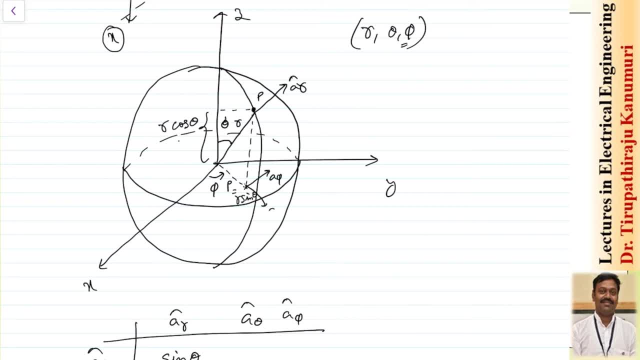 this. This is my direction of a phi, This is my direction of a rho, And the ar will be in this direction When you are projecting. it will be in the direction of a rho, but it is 90 degrees perpendicular to a phi. 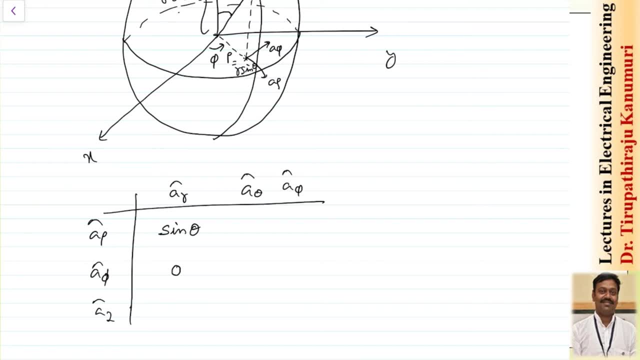 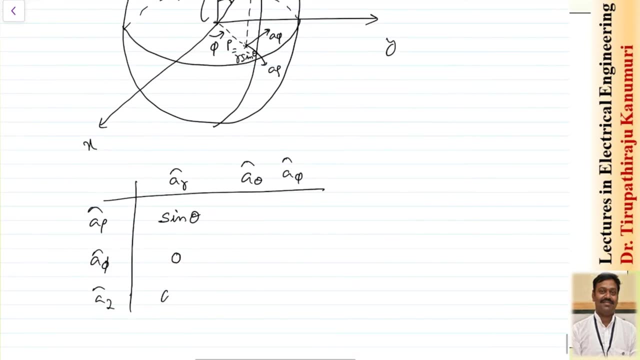 So automatically this component will be equal to 0.. So up to here it is clear. Now, coming to the z component: Z component we have already seen we can get for using cos theta. So that is why this will be equal to cos theta. r is done. Now let us complete for the case of phi. So for a phi. 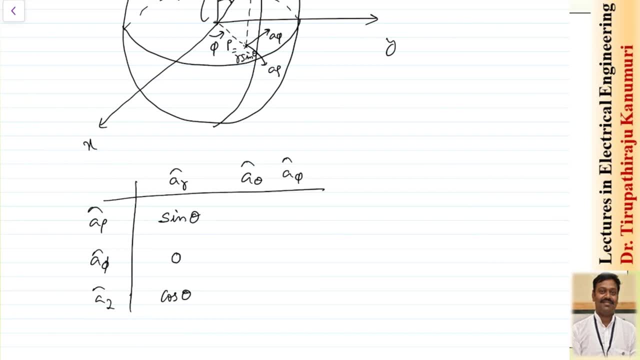 because a phi is perpendicular to a rho, because a phi is available in this cylinder we can get for using cos theta. So this will be 0,. this will be 0.. a phi dot. a phi will be equal to 1.. Now only a theta is remaining. How to remember the value of the theta? You can see here: 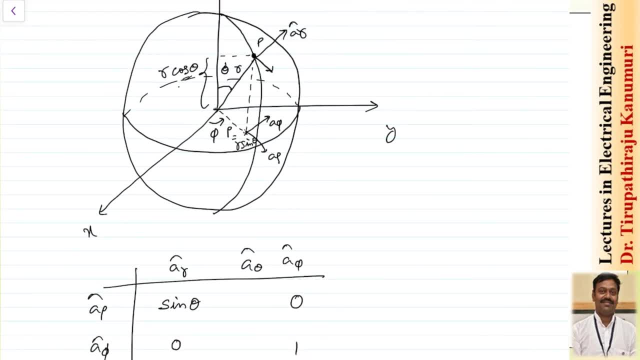 the incremental value of the theta will be in the incremental direction. So this is my direction of a theta. So let me try to draw it here so that it will be more clear to you. So x, y and z, this is my radius, having an angle of theta here, the direction of a theta. 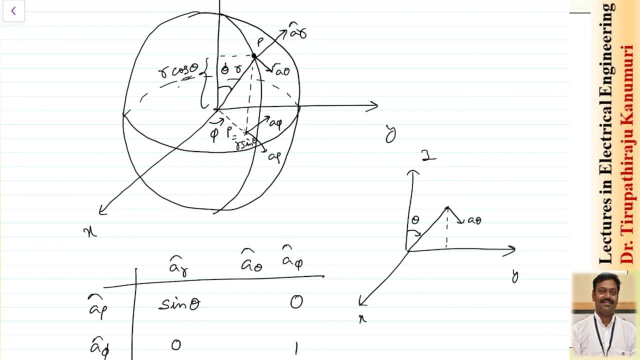 So for this what I am doing, I am just drawing a vertical line and a horizontal line, So this forms 90 degrees. Remember here, as it is a tangent, at this point this angle will be 90 degrees. So 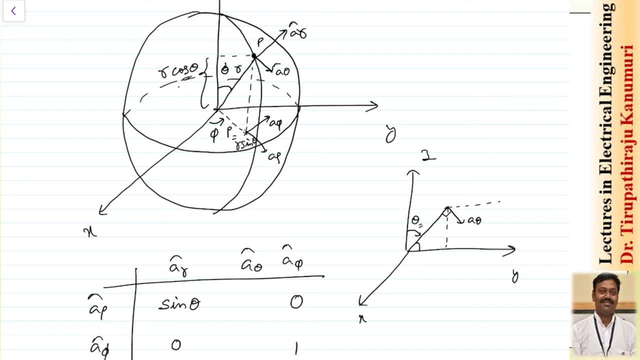 this angle is theta, The total angle is 90 degrees. So this will be equal to 90 minus theta. So this angle is 90 degrees. So obviously this angle will be theta. So when this angle is theta, 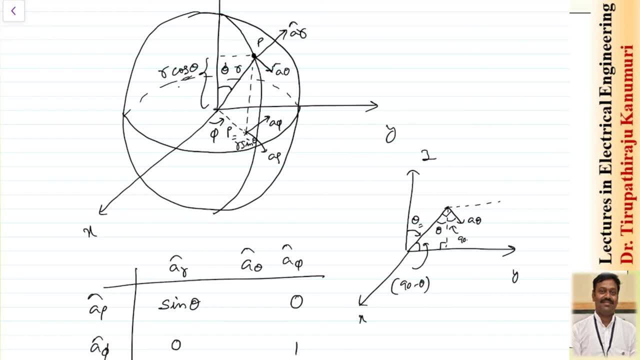 so what will be this angle? This angle will be 90 minus theta. So obviously this angle will be theta. That means a theta you can project in the direction of x, y plane, That means in the rho plane, And second one, it can be projected in the direction of the z plane. So it will come. 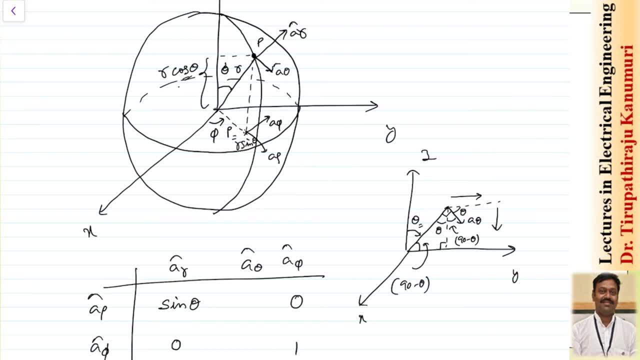 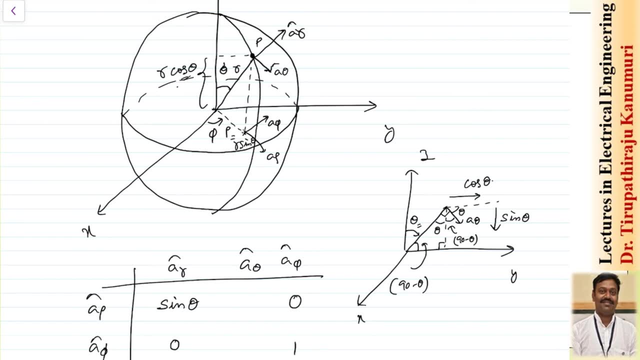 like this. So this will be a theta. You are resolving in the sine component, So this will be equal to sine theta. This will be equal to cos theta. That means if you are taking the cos theta, it is projecting in the x? y plane or the rho plane. So that is why a theta in the direction. 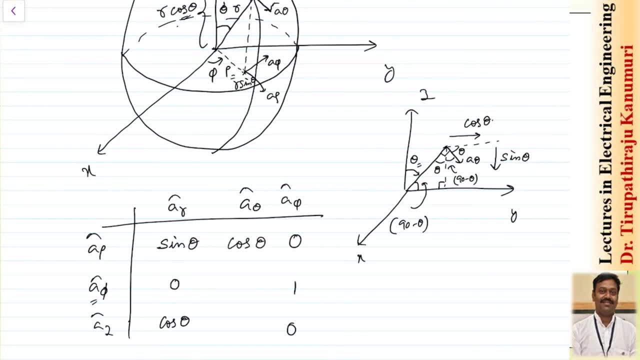 of rho will be equal to cos theta. Then a theta in the direction of x y plane will be equal to cos theta. direction of phi. a theta in the direction of phi, because a theta and phi are 90 degrees here, because in this coordinate they are 90 degrees. so this will be equal to 0. now in the z direction. 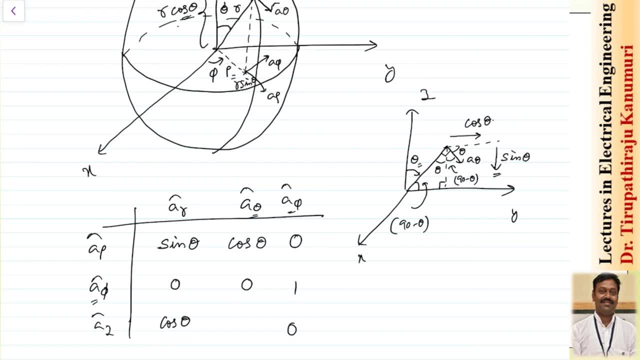 you can see, here this arrow is showing opposite direction to direction of z. that's why you have to take minus of what is coming here, so this will be minus sine theta. so i think this is clear to how to convert between spherical to cylindrical and vice versa in this way. we have to do it so. 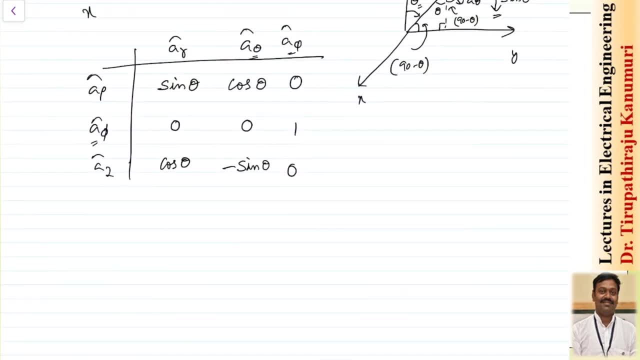 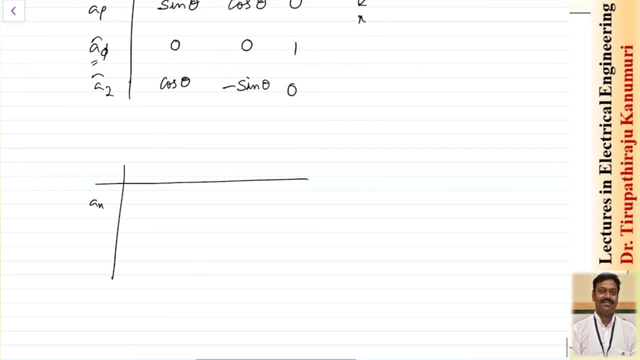 let us see how to convert between rectangular coordinate system to cylindrical or spherical coordinate system, and vice versa. so for that again, i am taking the table. so take it as ax, ay, az. this will be ar, a theta and a phi. these are the different things. so let us try to calculate. 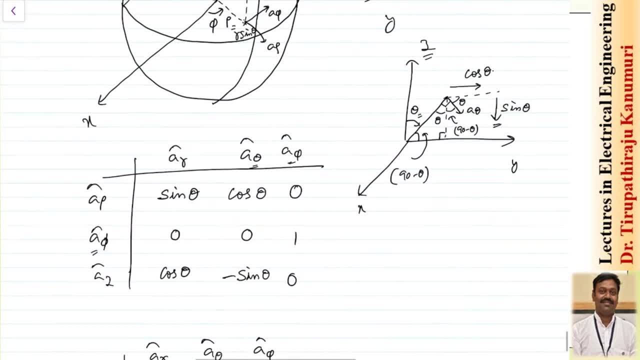 one by one. first one is: first, let us take ar. so ar, i have told you this. ar, when you are projecting in the xy plane, first we have to think about the distance between yz and the rz is equal to the yz is equal to the primeira chance that we are representing. similar if the given yz value. 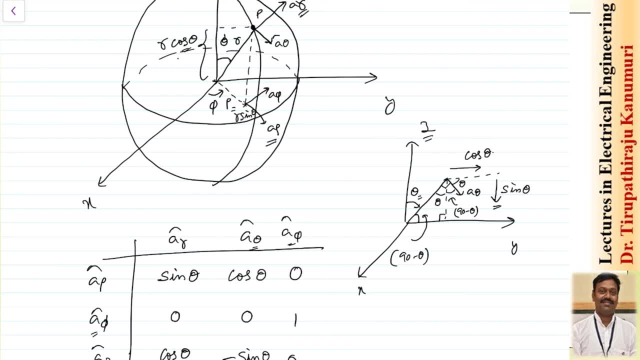 the rr of the paved slope is Μy is equal to the kya問題. so when we do the construction of this data be projected in the direction of the row or the xy plane, now in the, when it is projected in the xy plane, it is multiplying with sine theta. we have just seen there ar when it is projected in. 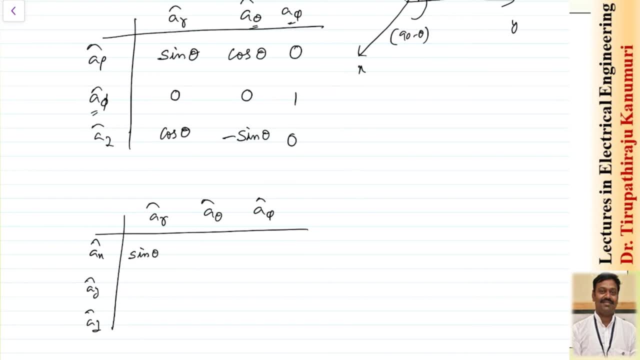 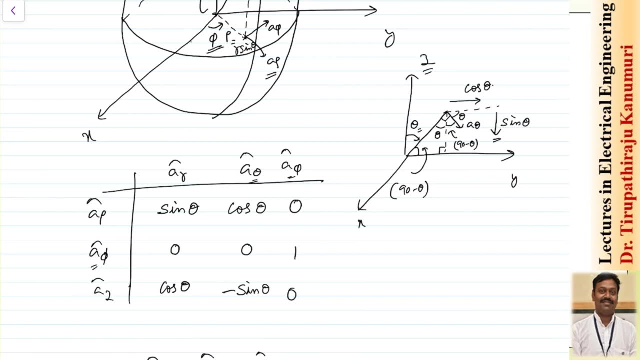 the row direction, it becomes sine theta. so this sine theta or the row, if you want to convert from this row to the x direction, we have to multiply with cos phi, because when you are projecting this to the xy plane we have to take it as cos phi. we have seen in rectangular to cylindrical. 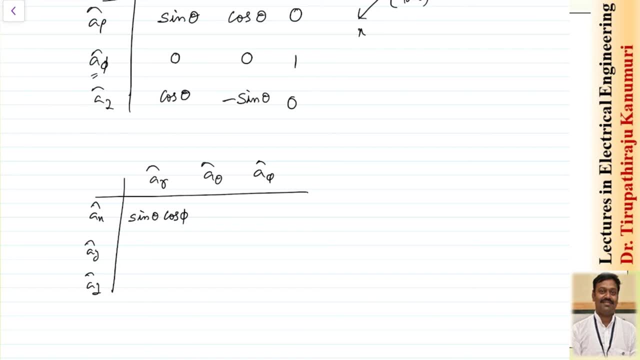 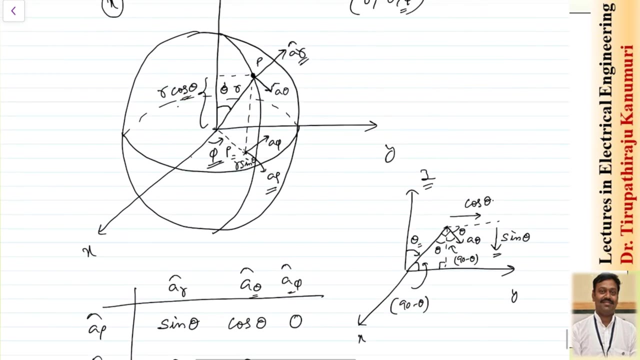 coordinate conversion- so this will become equal to sine theta- into cos phi and second one: this will be sine theta. you have to multiply with sine phi to get the y component. then ar in the direction of z. so ar in the direction of z. we have already derived here this ar in the direction of. 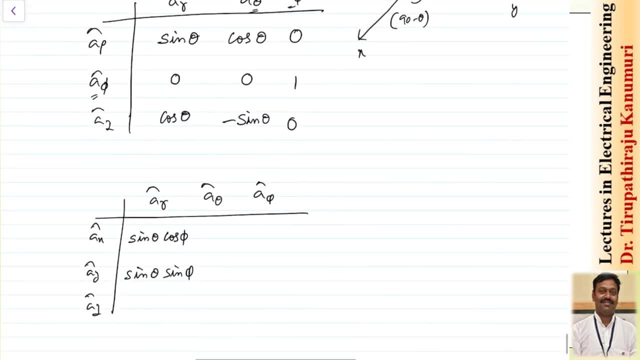 z is obtained by taking cos theta, so that is why i can write it as cos theta. this part is done, so let us complete for the case of the a phi, then we will go for a theta, because a theta is little complex, complex, So here it becomes little bit tight, so I am just erasing it. 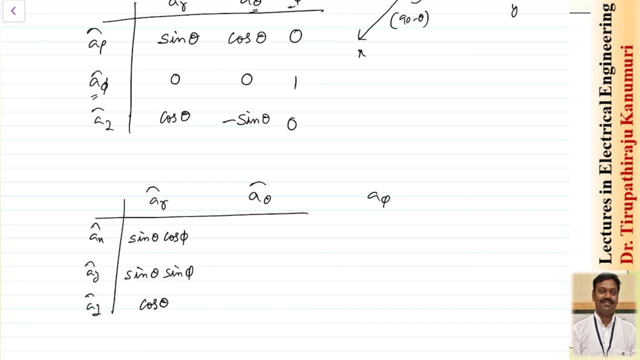 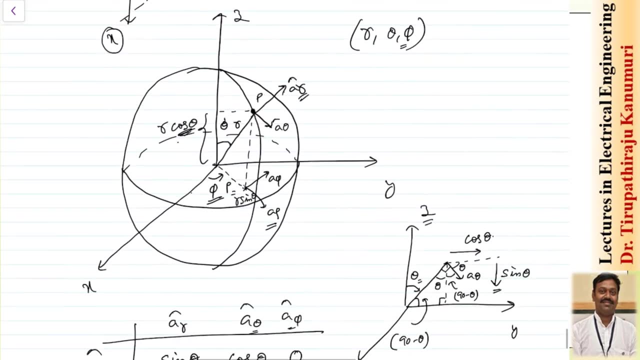 This will be equal to a theta. then this will be equal to a phi. So let us take the value of a phi. Now coming to the value of the phi, coming to the value of the phi. so the phi I want to convert to x, y and z coordinate. 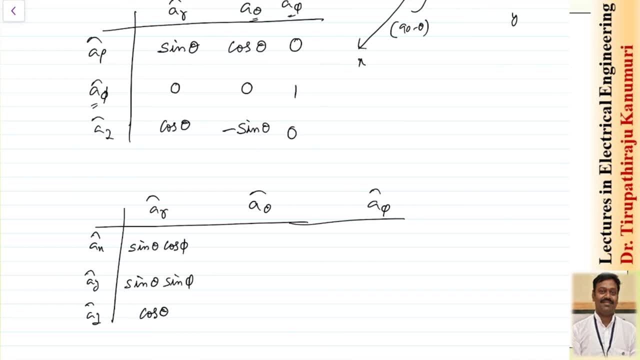 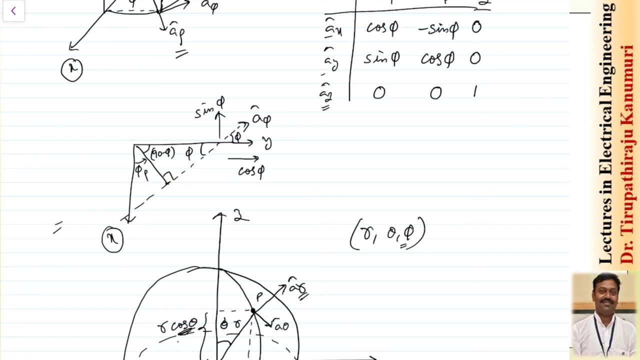 This phi is same as in the cylindrical coordinate system. So whatever we have seen for the cylindrical coordinate system, the same thing can be kept here In cylindrical coordinate system. we have drawn this diagram. So from this diagram we got that the cos phi will be y component and sin phi will be. 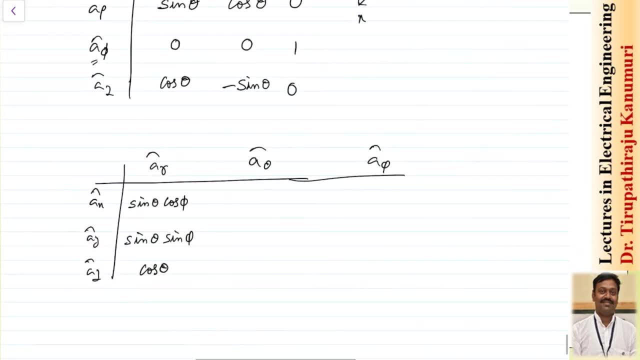 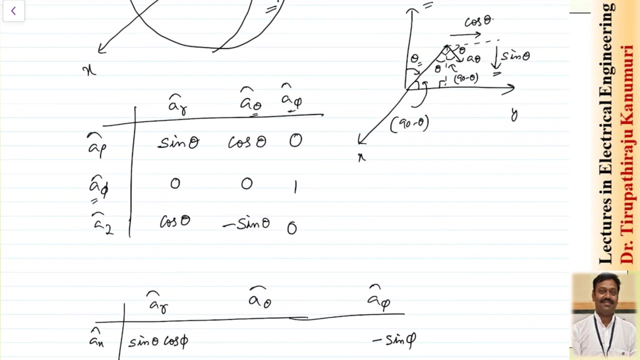 minus x component. That means x component will be minus sin phi and y component will be cos phi and z is perpendicular to theta, so it will become equal to zero. Now theta is remaining. Now coming to the theta again- we have seen here theta- the xy plane component will be: 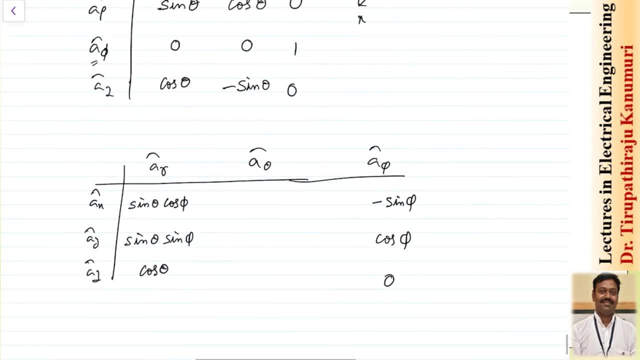 equal to cos theta. That means xy plane component is equal to cos theta. If you write cos theta it will convert to the xy plane. So that xy plane should be shifted to x. that means it is in the row plane. So to shift in the x direction I have to multiply with cos phi. 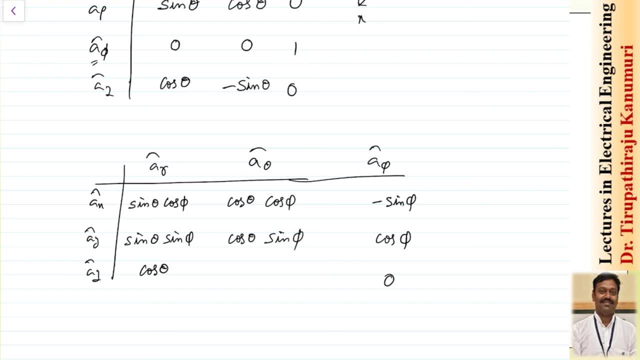 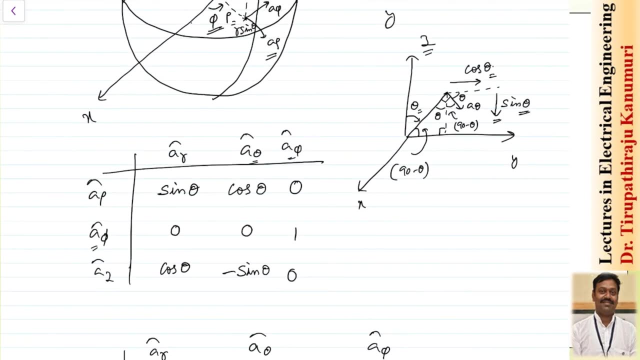 So shift in the y direction. I have to multiply with sin phi. So up to here it is clear to you. Now, coming to the last component: a theta in the direction of z, a theta in the direction of z. you can see we are getting sin theta, but it is opposite direction to z. 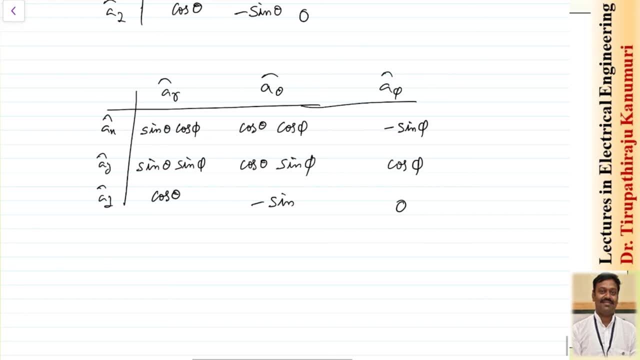 So this will be equal to minus sin theta. So once you were able to draw that table- what is required in the exam? using these relationships you can solve the numerical easily. So here I briefly discussed about the things and the numericals and other things I have. 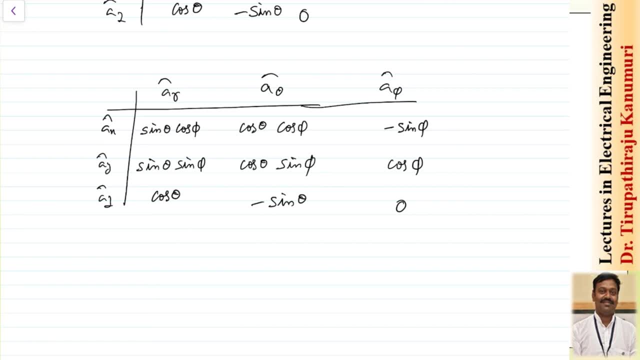 already discussed in my previous lectures. You can try to summarize this by taking any numerical and try to solve it. If you still have any query, you can leave your comments in the comment section below. I will answer to your queries from there, Thank you. Thank you very much. 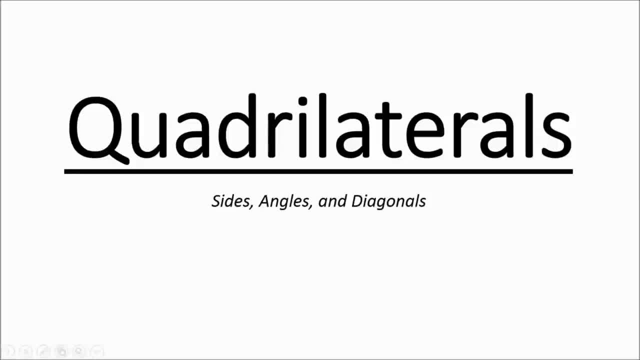 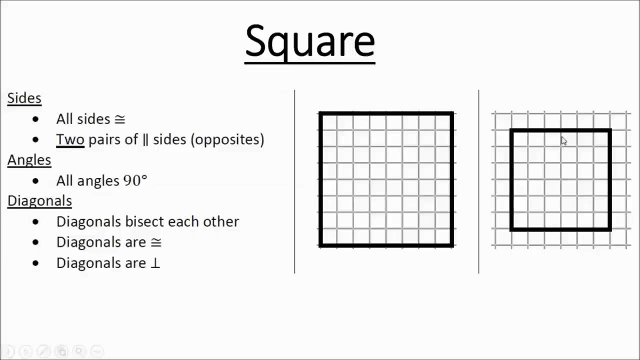 So this video is going to cover quadrilaterals and it's going to describe different quadrilaterals by looking at the sides, the angles and the diagonals. So our first one's a square. We've got two pictures of squares. Now what we're going to do is I'm going to read the descriptions on the left and I'm going to mark the different pictures with different ways you might see it, to show these characteristics, or also known as these attributes. 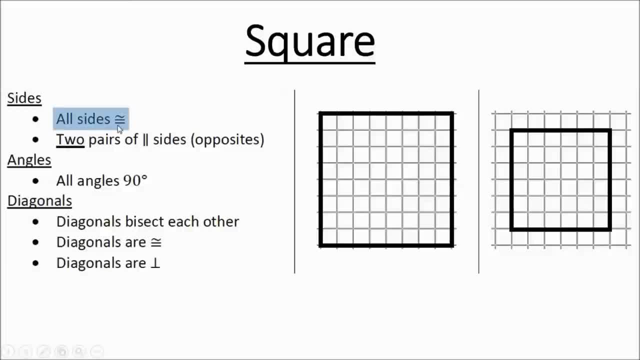 Okay, so all sides are congruent. That means having the same measurement. So over here we're going to have these sides with single slash lines in them, showing that they're all the same measurement. When you see single slash lines in all of those sides, all of those measurements are the same. 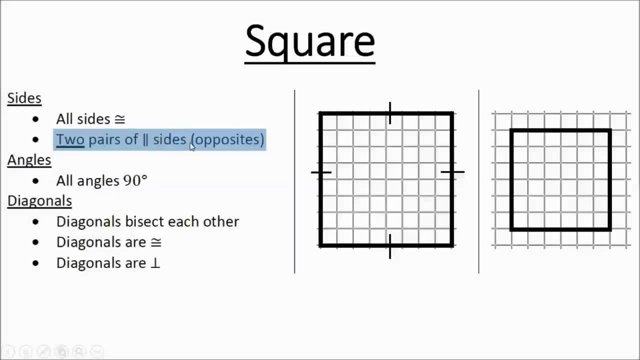 Also, you're going to have two pairs of parallel sides, the opposite sides being parallel. So over here we'll have these two sides. They're opposite each other, They're parallel, And then the top and bottom sides are also parallel, And that's how you'll see them marked with these different types of arrows.